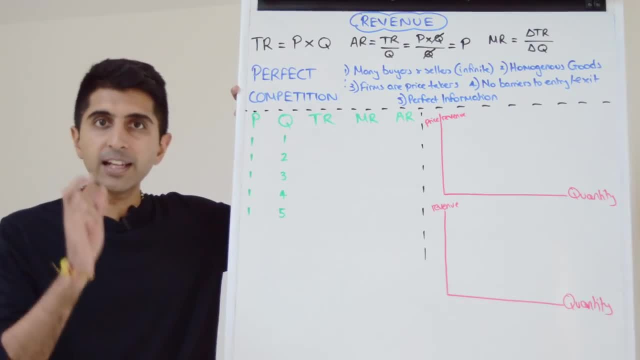 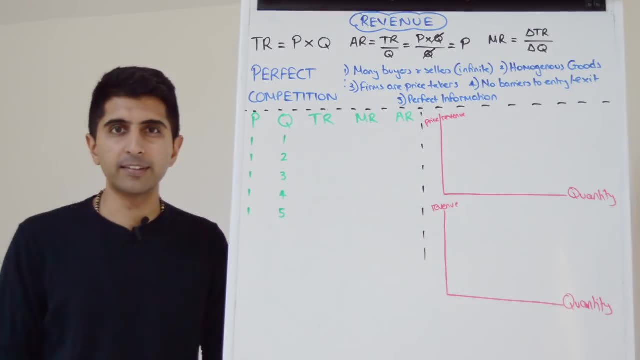 there. Well, we need to understand what the characteristics are of a perfectly competitive market first. In this kind of market, there'll be many buyers and sellers. if I'm being precise, infinite buyers and sellers. This is a very theoretical extreme market structure- insane. 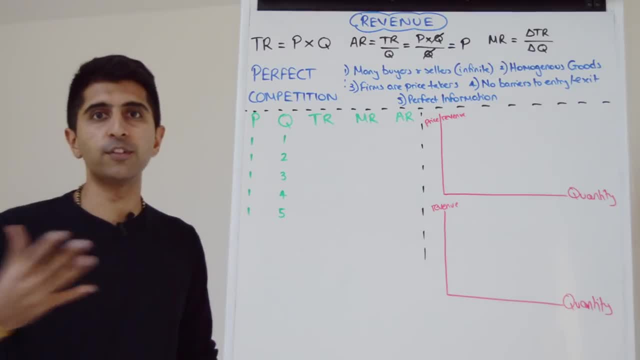 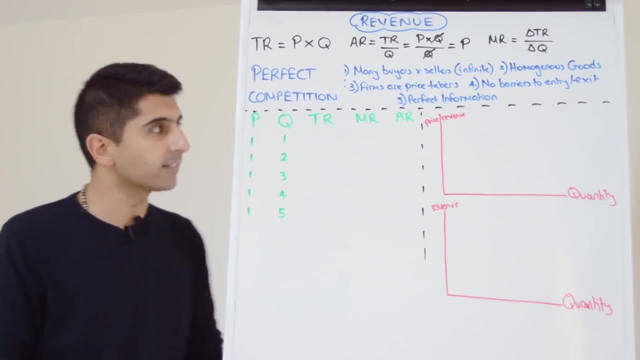 intense competition. All these firms are selling homogenous goods and services, meaning identical goods and services, and that means that these firms are price takers. They have no ability to set their price. they have to take the price in the market and charge that price. There are no. 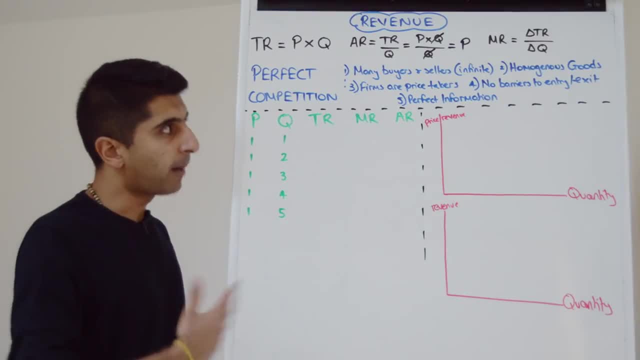 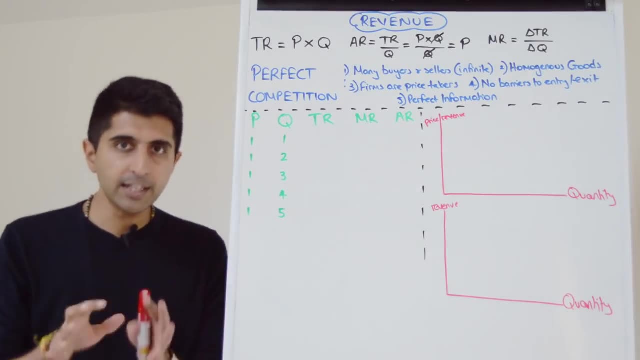 barriers to entry and exit and there is perfect information of market conditions. No barriers to entry and exit means free movement in and out of the market. Okay, so we get the basic idea: insane competition. What does that mean in terms of revenue? That's what we're looking for. Well, 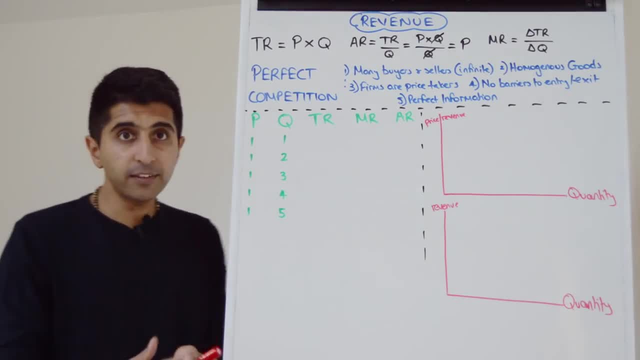 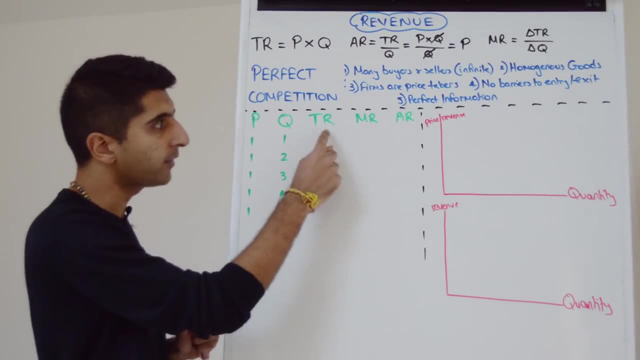 it means this firm is a price taker, crucially So, regardless of the number of units they're selling, they're always going to be selling them at the same price. So let's say the price is a pound and here are the units they are selling. Let's work out TR, MR and AR using our equations above. 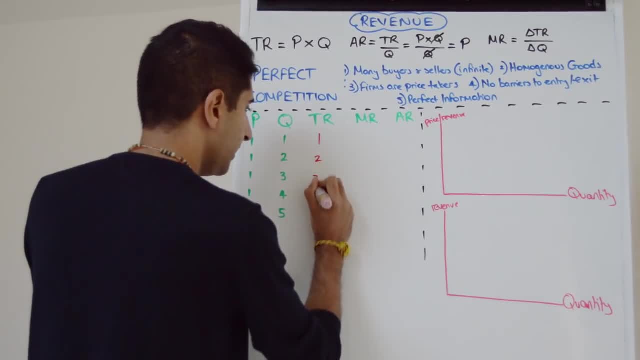 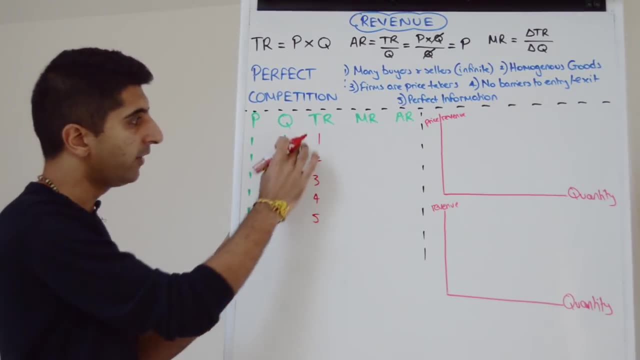 TR is P times Q, so we're going to get at one, two, three, four and five. so we say this is in pounds or dollars. whatever marginal revenue is the change in TR divided by the change in Q. the change in Q is always one. so we're just looking at the change in TR, which in each case is: 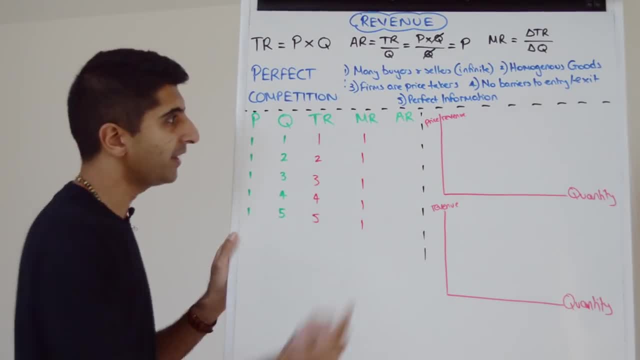 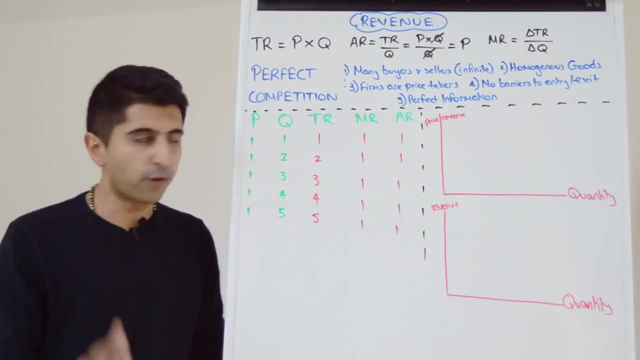 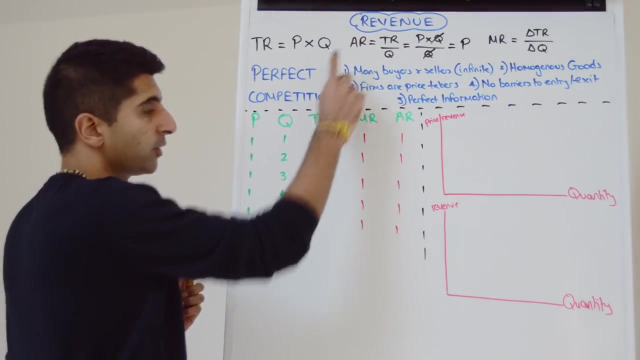 one easy stuff and average revenue. look at, the trick is just price, so that's going to be one as well. okay, that's great. so if we see the numbers here, it's very easy now to draw our revenue curves. let's start by drawing average revenue and marginal revenue. we've got to have price and revenue on the axis because 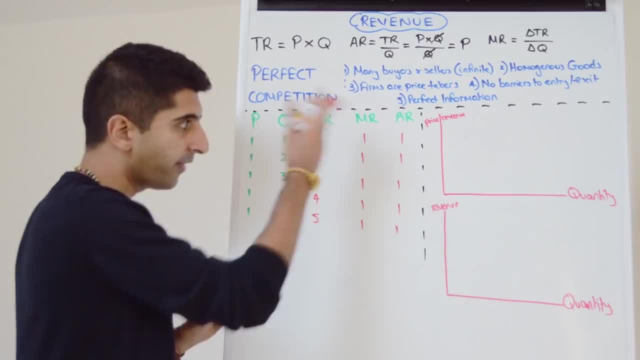 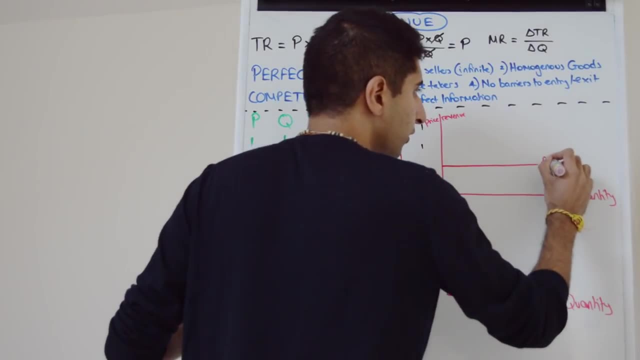 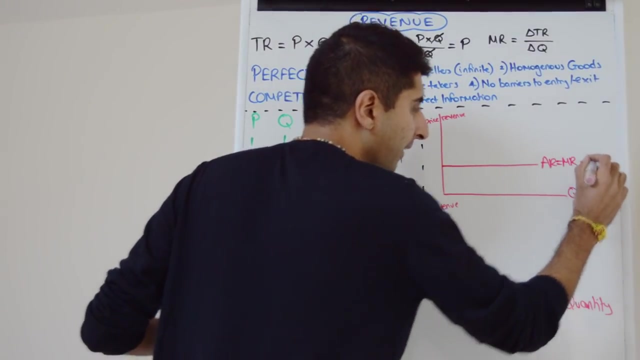 we're drawing AR here, but we can see that both AR and MR are the same and they are constant over a range of quantity. so AR and MR in perfect competition will just look like that. but I'm not going to stop my labeling there. I'm also going to say: AR equals MR, which equals demand, and at the end of this, 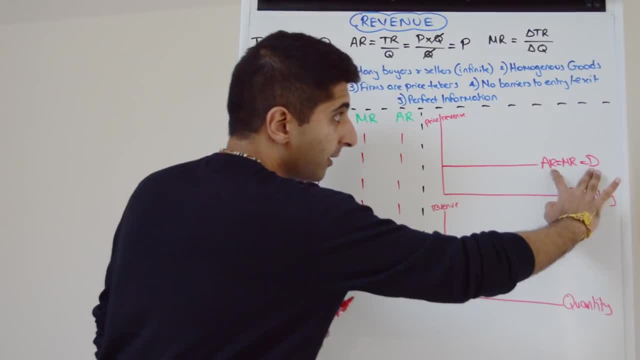 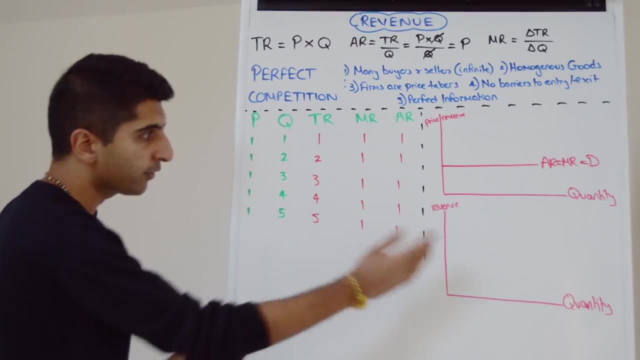 video I'll explain why average revenue is equal to demand. that will come later, but there we go. that is very simple, and if I had to put a figure here, that figure would be one pound there. what about total revenue? we can see that total revenue is increasing, but always increasing by one. so therefore, if 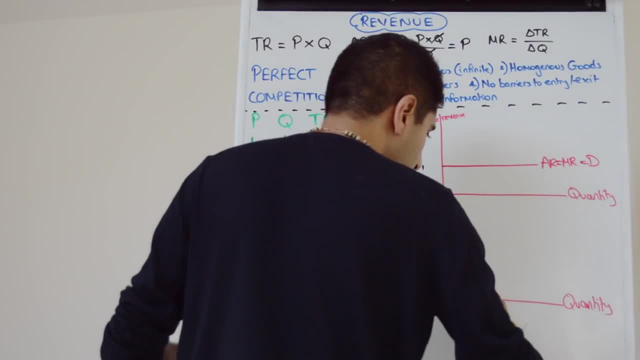 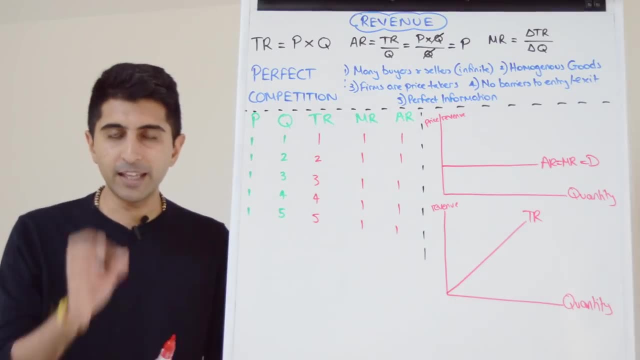 we're drawing our total revenue curve. it's going to be a linear upward sloping line showing a constant gradient, always increasing by one. so very simple: revenue curves in perfect competition, easy, as you like. what about when there is imperfect competition? how do our revenue curves change there? well, imperfect. 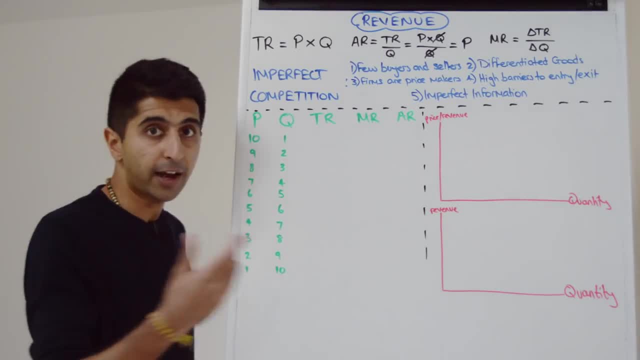 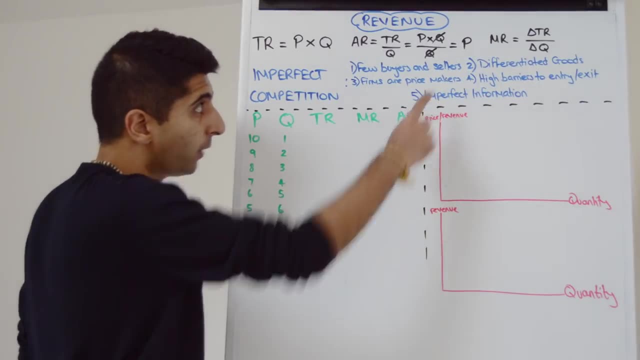 competition is the exact reverse of perfect competition. let's look at the characteristics. so now there are few buyers and sellers. they're all selling differentiated goods and services, making them price makers now, so they can set their own prices. there are high barriers to entry and exit, and 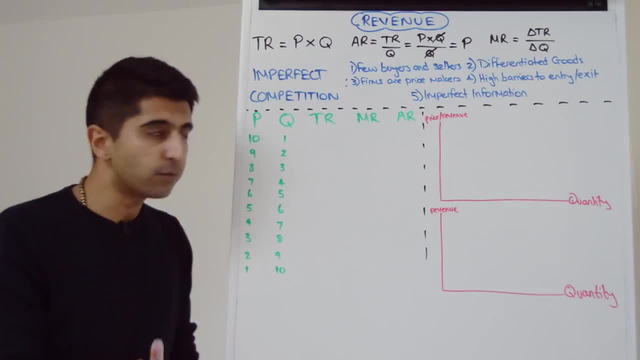 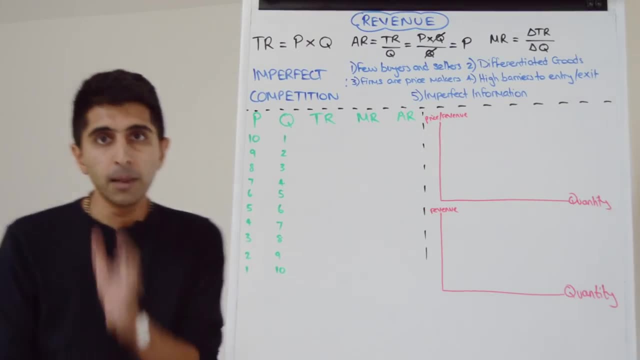 there is imperfect information of market conditions. everything in reverse. here the key thing is that firms are price makers and we can see now that we've got different prices being charged by the firm. but crucially, they are going to be governed, these firms, by the law of demand, so high prices, quantity sold is. 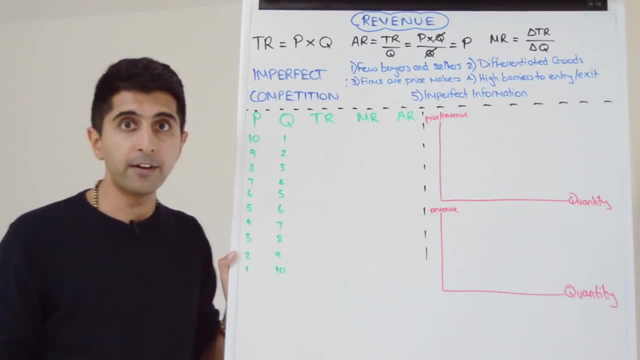 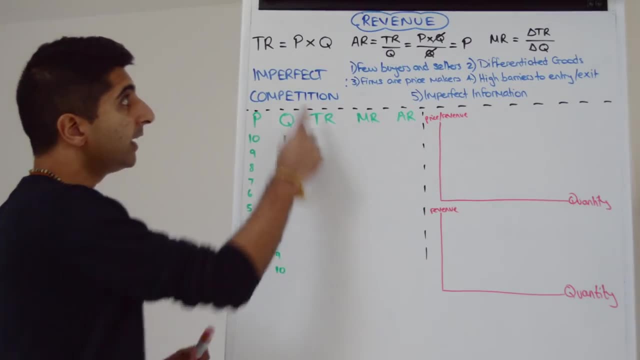 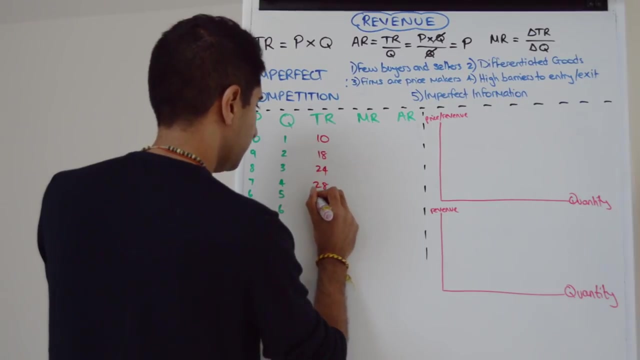 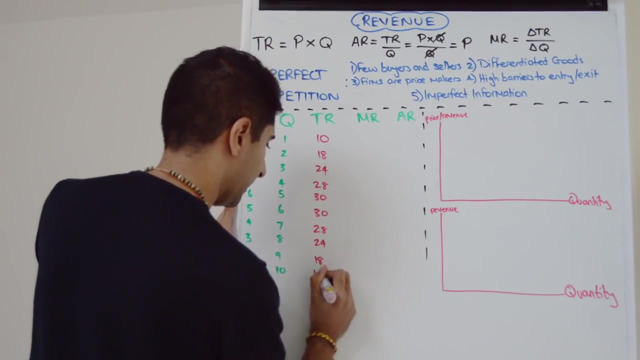 going to be low and at low prices. quantity sold is going to be higher, right, but we want to focus on revenue. that's what we're here for. so let's calculate TR, MR and AR given these figures. here, TR is just P times Q, so we're going to get 10, 18, 24, 28, 30, 30, 28, 24, 18 and 10. very. 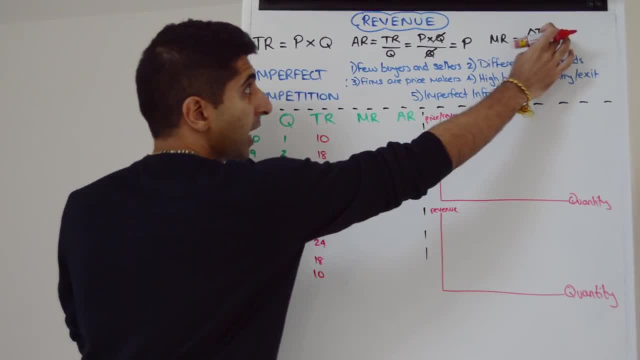 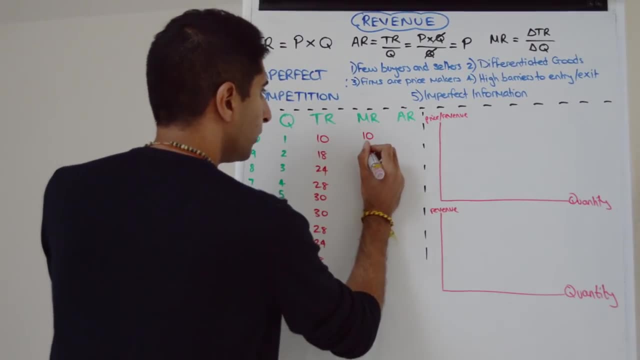 simple: P times Q in each case. let's do marginal revenue, which is the change in TR, over the change in Q. the change in Q is always one. so that makes our life very easy. we just have to look at the change in TR. so you have 10, then we go to 8, to 6, to 4, to 2 to 0, and then MR can go. 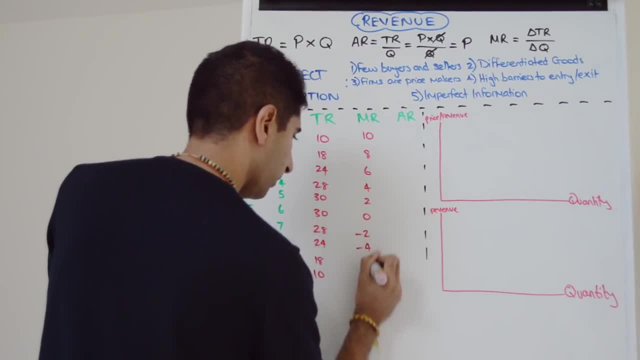 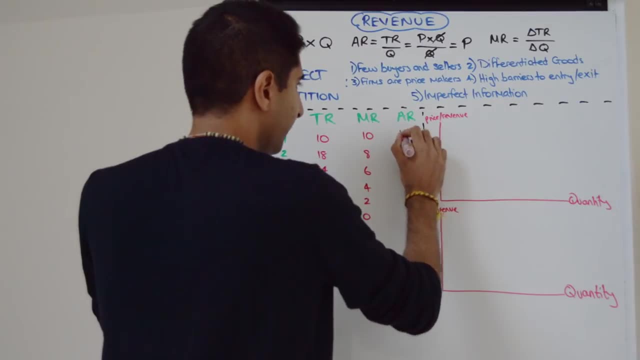 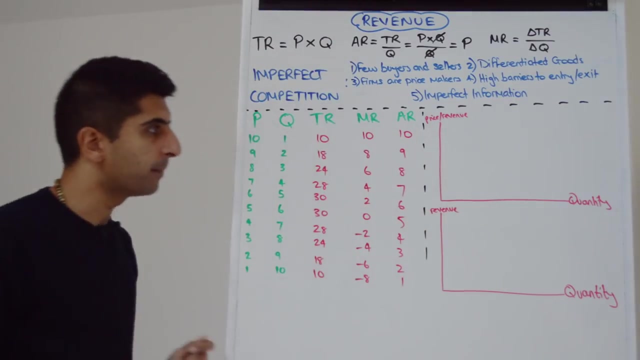 negative and it does here to minus 2, to minus 4, minus 6 and then minus 8 to finish. average revenue is just the price. that's our little trick, lovely trick. so you just have 10, 9, 8, 7, 6, 5, 4, 3, 2 and 1. really simple stuff. using these numbers. 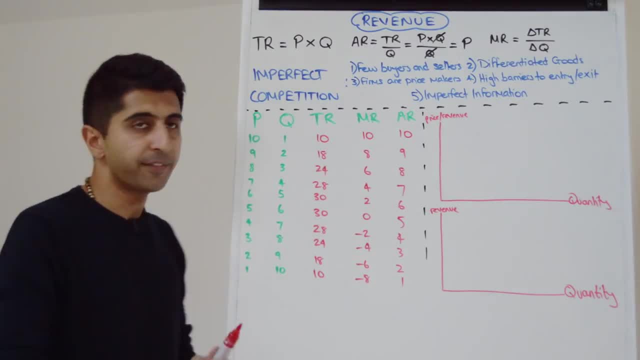 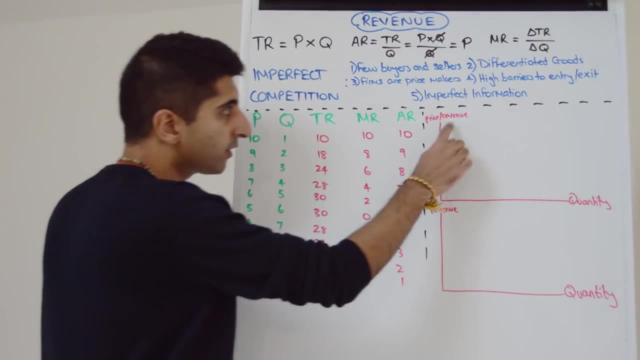 we could plot the curves. I'm not going to plot, I'm going to use these numbers to give us a general shape of the curves. what I want to draw first is our average revenue curve, and we can see that average revenue starts high and then it falls. doesn't it remember? average revenue is just a demand curve and if we 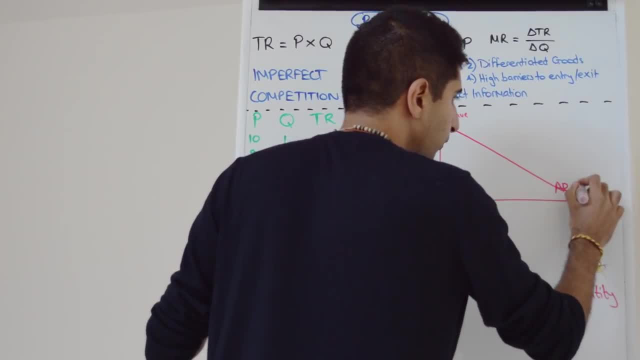 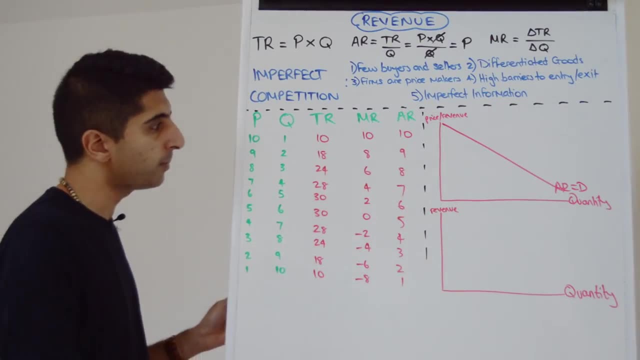 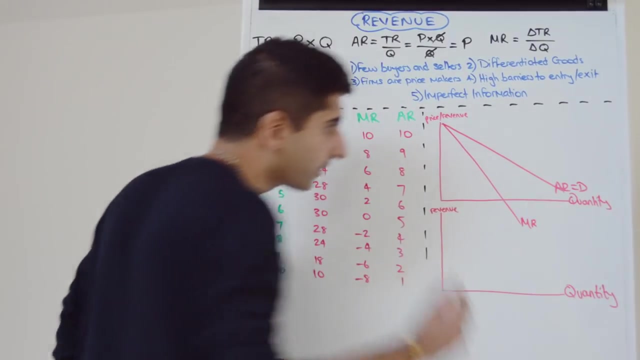 draw it, it looks exactly like a demand curve that we are used to. okay, great. what about marginal revenue? marginal revenue starts at the same point and also decreases. it's also downward sloping, but, you can see, at a much faster rate than average revenue negative. so marginal revenue is going to look like that precisely. marginal revenue is twice. 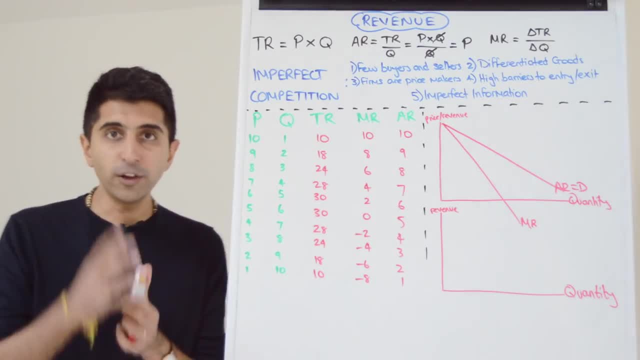 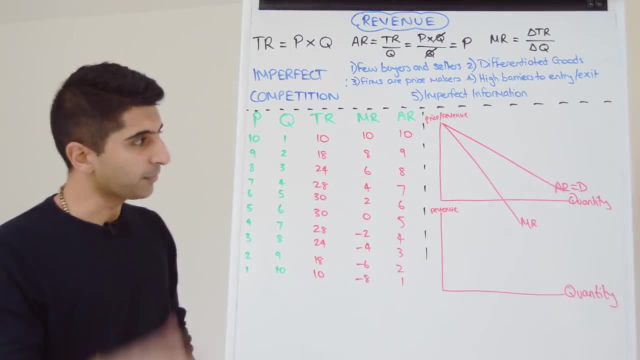 as steep as average revenue. there are two ways to understand that. one is with the mathematical proof. if you click on this link here, guys, i have done that proof in a different video. you can watch that. it's very interesting. that's probably the best way to understand it mathematically but intuitively. look at it this way: when a firm drops its price, it's not just dropping its price for the next unit sold, it's dropping its price on all the units that it's selling. even the units that it sold beforehand are now being sold at a lower price, and that means that marginal revenue is going to. 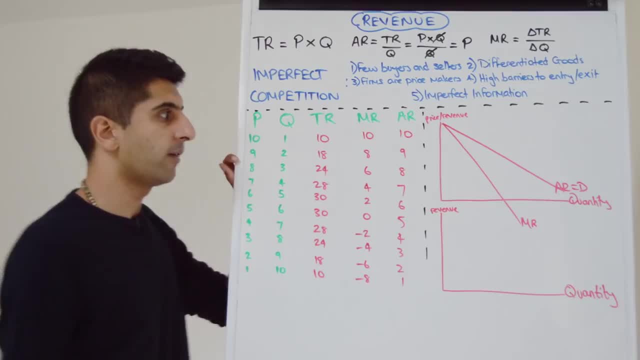 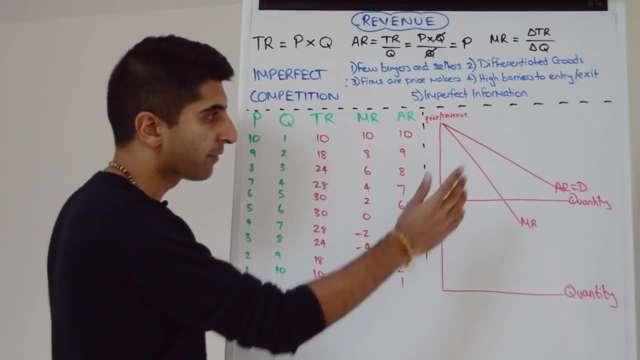 drop twice as steep as average revenue. it's going to drop faster than average revenue, but you don't need to know the the um, the detailed logic there at all. just make sure you draw it roughly twice as steep as average revenue. okay, while we're here, why is average revenue equal to demand? 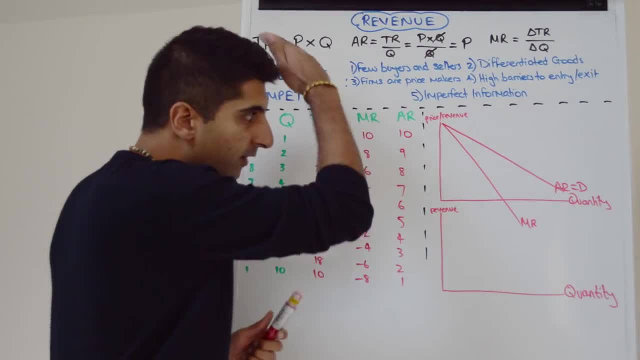 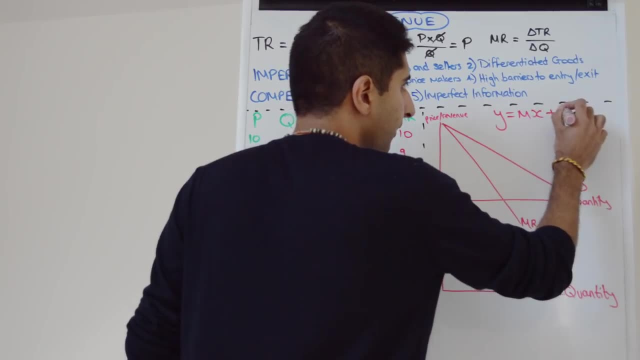 this is important here. right, let's look at demand. demand is just a downward sloping linear line and all linear lines take this form from maths, if you remember: y equals mx plus c. that's the basic equation of a linear line. okay, where c is the y intercept, m is the gradient, it's. 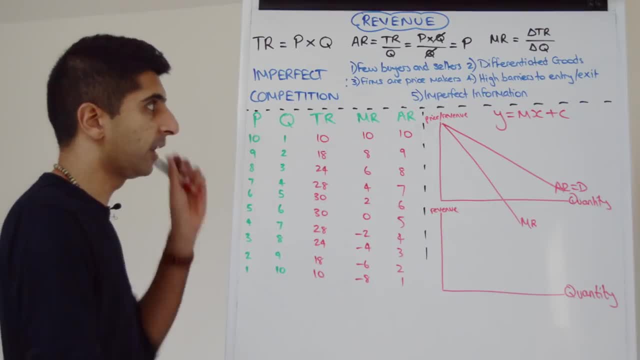 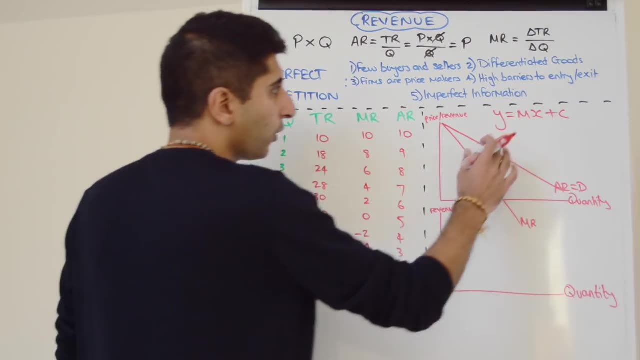 the coefficient of x. so m is just the gradient right, the slope of the line. okay, fine, our demand curve is downward sloping. it's a linear line, all right, but let's apply it now to this form. so y is price when we draw a demand curve, isn't it? so we can say price equals. let's take our y intercept. 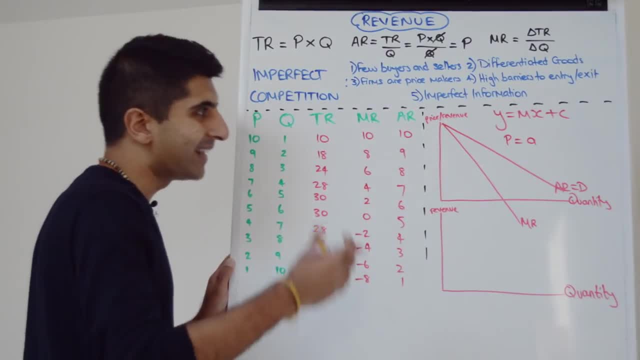 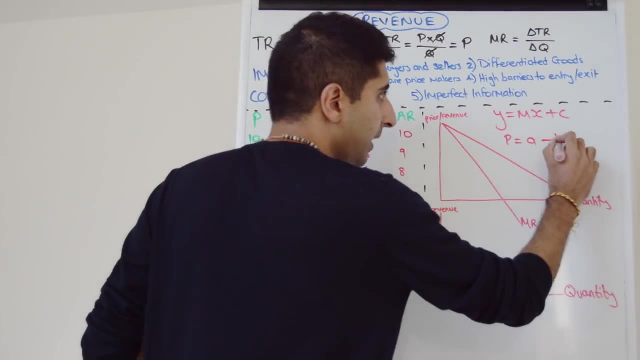 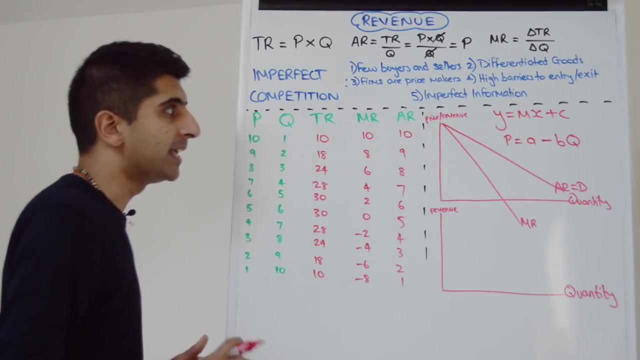 first, and let's call it a. so a is our y intercept and it's a negative gradient, so it's going to be minus. let's call that coefficient, that gradient, let's call it b, and on the x-axis it's not going to be x, it's quantity. so p equals a minus bq. that is our demand curve. just apply to the basic form. 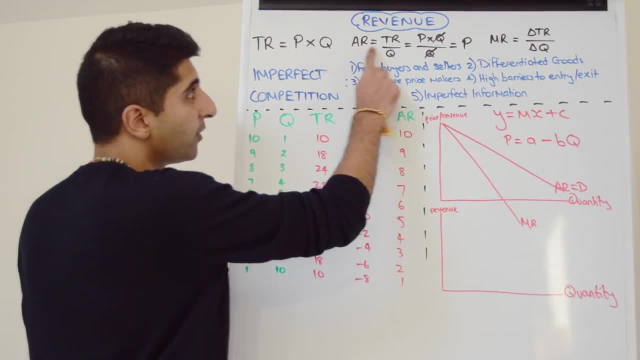 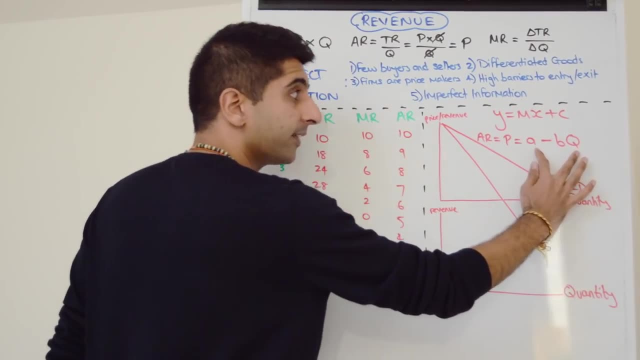 of y equals mx plus c. now we've just said that average revenue is equal to the price. so average revenue is equal to price. and if we're saying price is equal to this and this is our demand curve, it must follow that average revenue is equal to demand. there is no way you need to know that at. 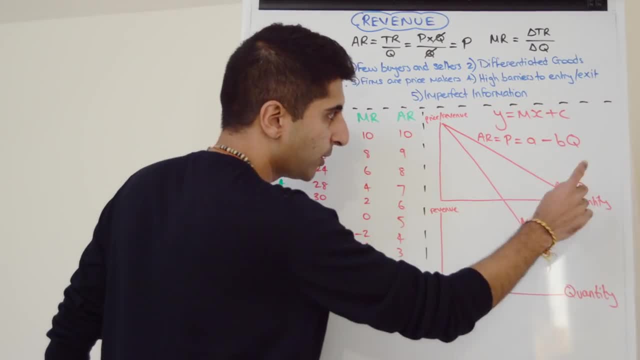 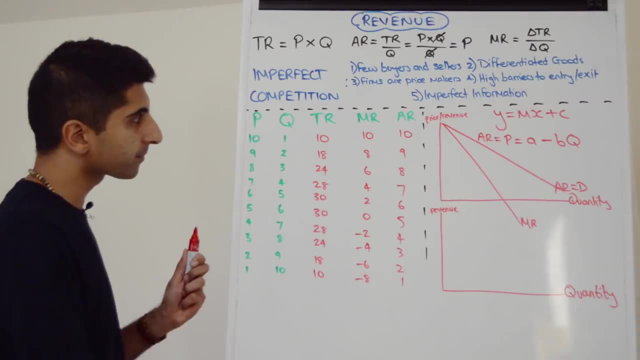 way, all you need to be able to do is to write down here that average revenue equals demand. but something of interest for you. no doubt you're asking that question beforehand. okay, great, what about total revenue? now? well, you can see, total revenue is rising, rising, rising, but at a slower. 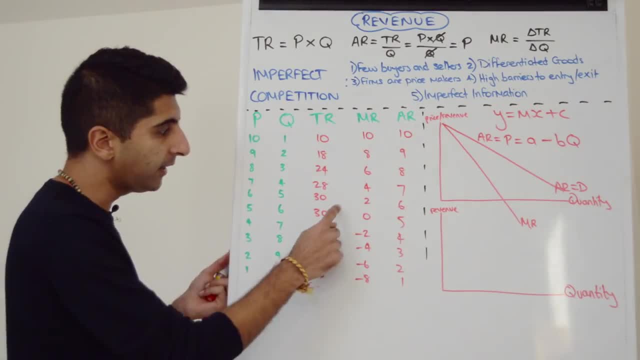 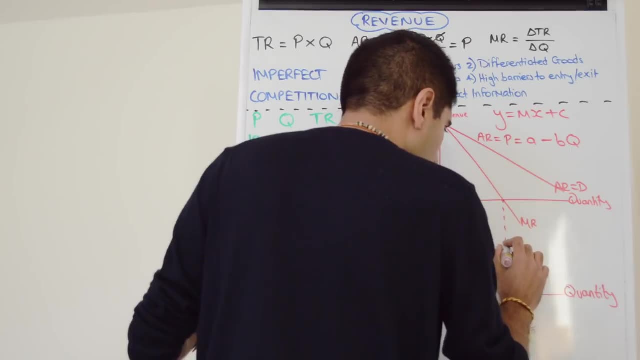 rate each time because marginal revenue is falling. it hits its peak and then it starts to decrease. okay, how do we draw that? well, we have to draw it precisely. total revenue will hit its peak where marginal revenue is zero. so it's going to be rising, but at a slower. 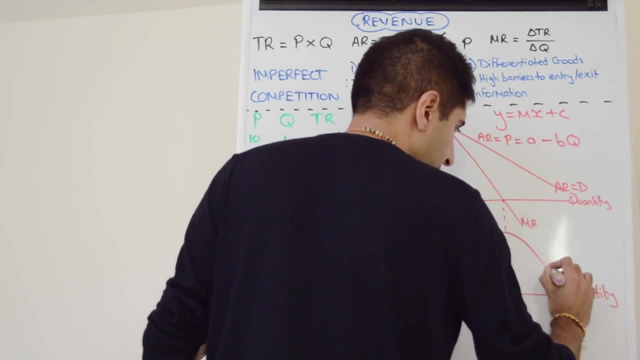 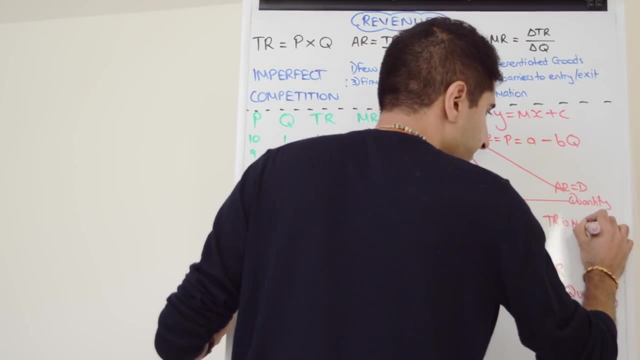 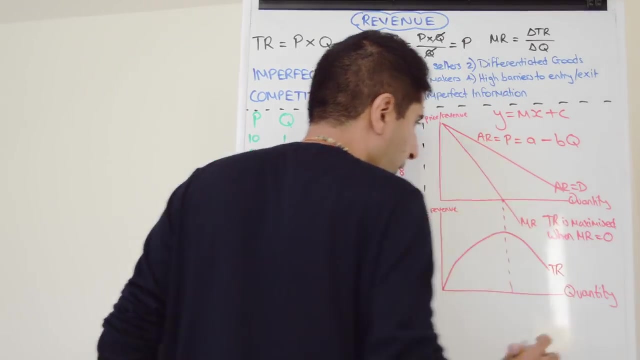 rate. it's going to hit its peak when marginal revenue is zero and then it's going to fall. there's our total revenue curve and we can write that on the side: that total revenue is maximized when marginal revenue is equal to zero. why is that? well, when marginal revenue is negative. 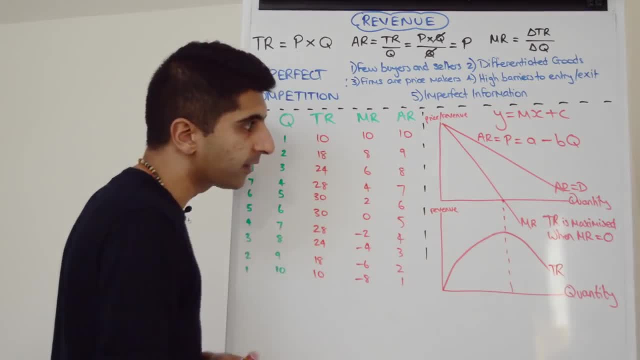 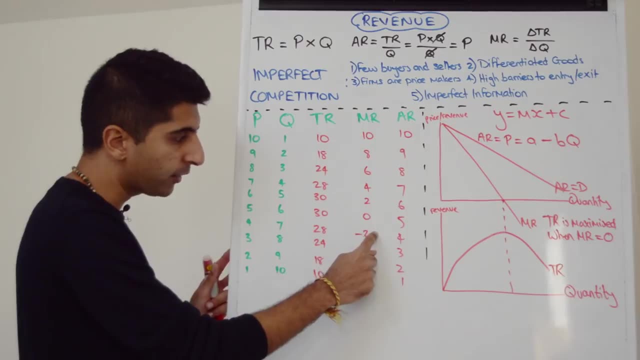 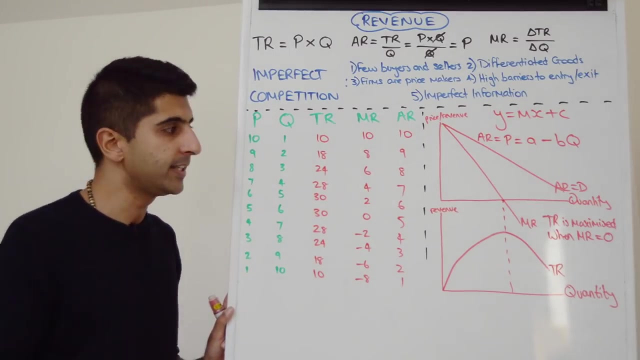 total revenue is going to be decreasing. all these extra units are being generated with negative extra revenue and therefore total revenue is going to come down. and we see that when marginal revenue is equal to zero. we see that very clearly here. when marginal revenue is negative, total revenue decreases. okay, fine. so any point to the right of where mr is zero cannot be maximizing. 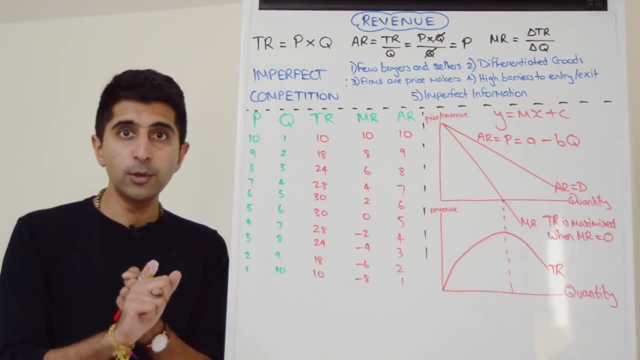 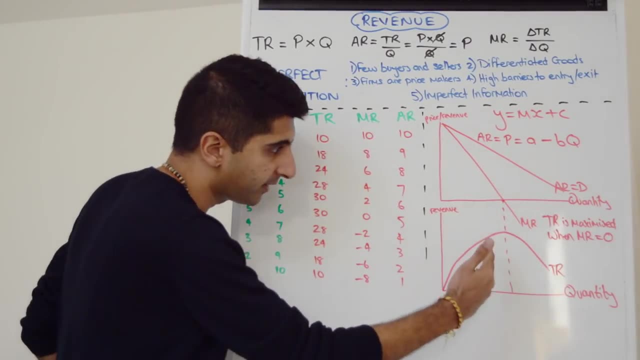 tr. any point to the left can't be either, because any point to the left. marginal revenue is always positive and therefore producing one more unit will always give you more revenue and therefore total revenue will keep rising. the rate at which it rises will be falling because marginal revenue is. 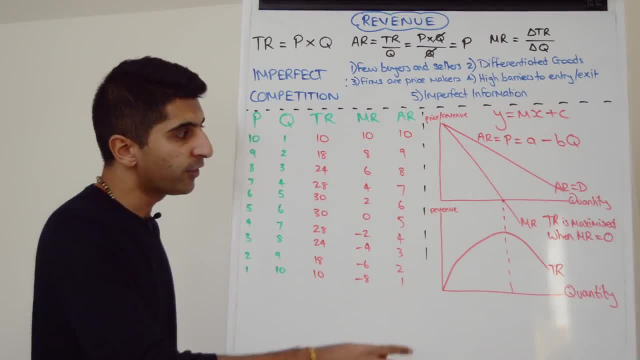 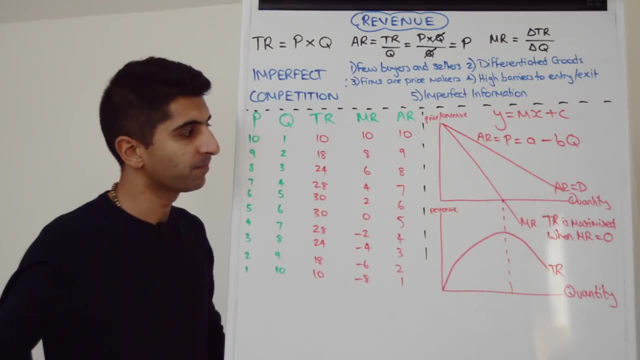 decreasing, but tr will always rise as long as marginal revenue is positive. only point where tr is maximized is when there is no more extra revenue to be gained, and that occurs where mr is zero. so that's everything you need to know, guys. that covers revenue curves in both. 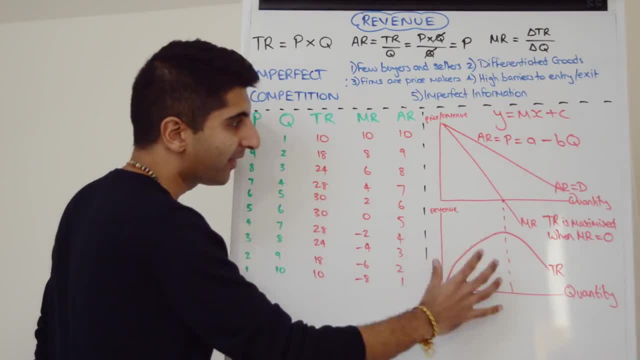 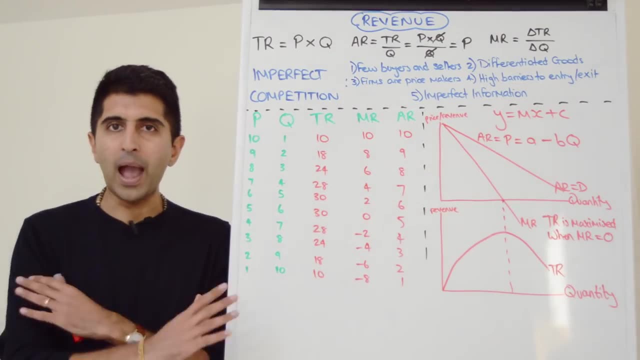 imperfect competition and imperfect competition. you can see that in imperfect competition, the curves look very different to how they looked in perfect competition. you've got the calculations, you've got the equations, you've got everything you need to smash this topic area. really hope you get it now. stay tuned for the next video. we're going to dive into profit now, putting costs and revenues. together and i'll see you in the next video. bye, bye. i'll see you all in that video. can't wait for it guys.